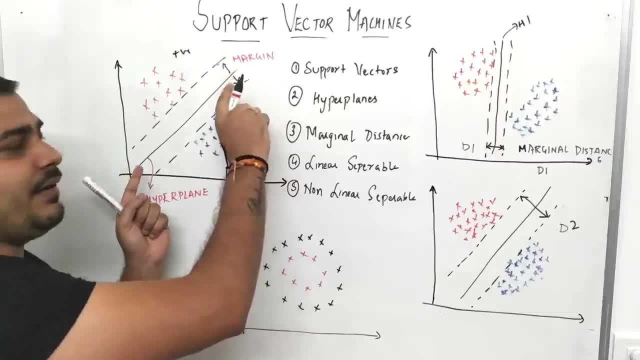 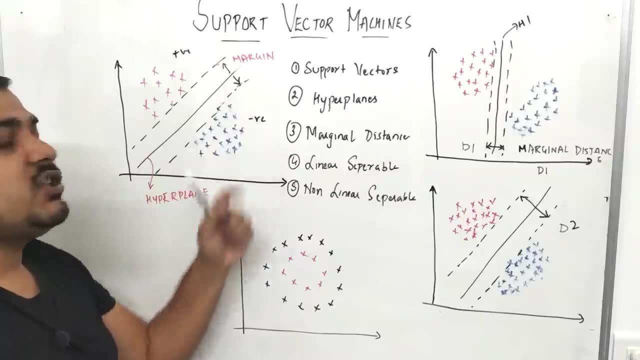 vector machine. make sure that when you are creating this hyperplane- right? so suppose this is my hyperplane over here. apart from this, it also creates two marginal lines, okay, and this two marginal lines will be having some distance, you know, so that it will be easily linearly separable. 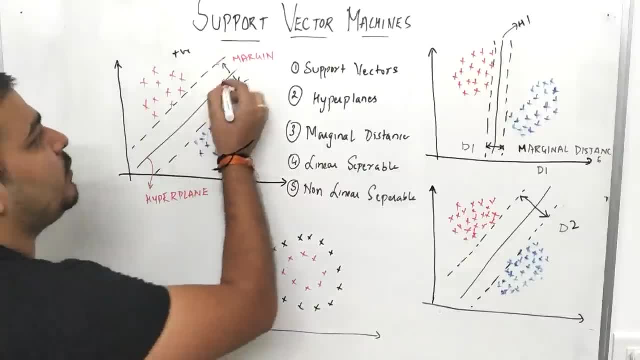 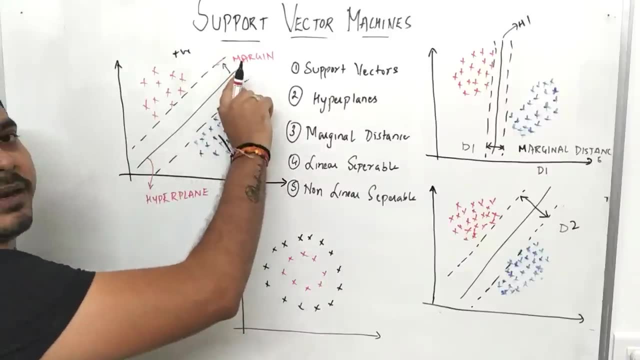 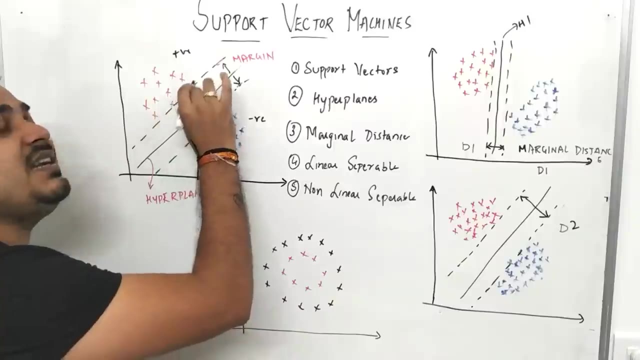 For both the classification points. right now. suppose, if I consider this hyperplane, it makes sure that there will be one more plane that will be parallel to this particular hyperplane and this particular hyperplane that you see, which is parallel to this one, right, it will be passing through one of the nearest positive or the negative point. so, after creating this, 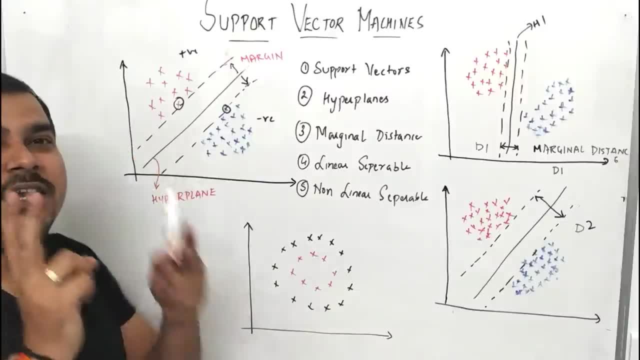 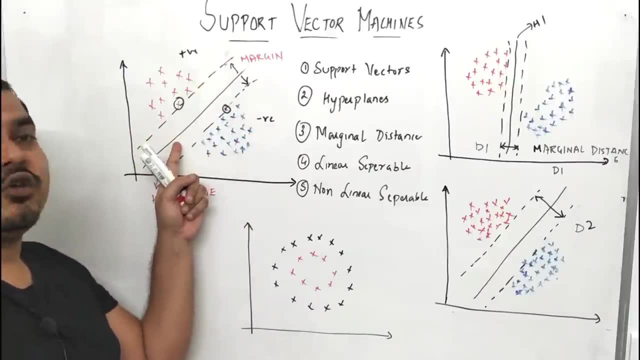 hyperplane. you know, what we do is that we also create two parallel planes, okay, the one in this dotted lines and the other one which is dotted line, and both- this particular line, will be parallel to the hyperplane that is actually created now, when we are creating this hyperplane. you know, this one dotted hyperplane which is parallel, 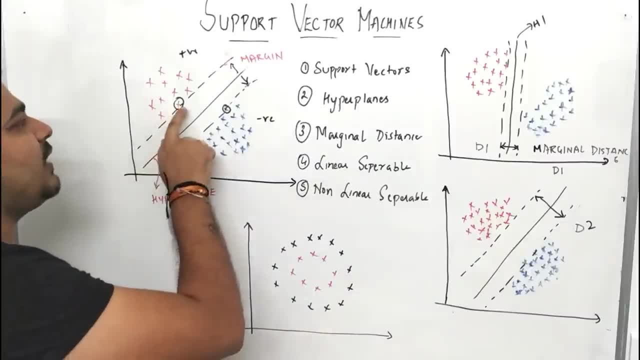 to the main hyperplane. over here we make sure that it passes through one of the nearest positive point. So over here this red one is one of the nearest positive point. similarly, when we are passing, we are creating the another hyperplane towards the negative direction. you can see that which? 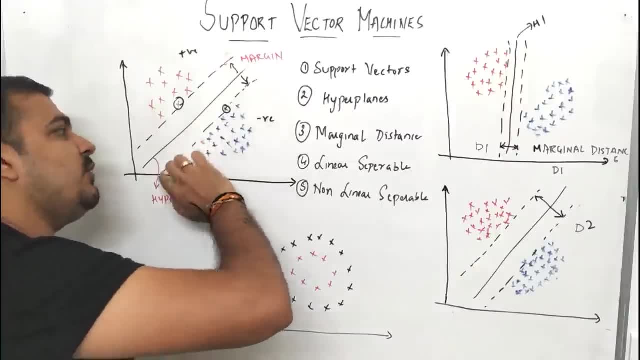 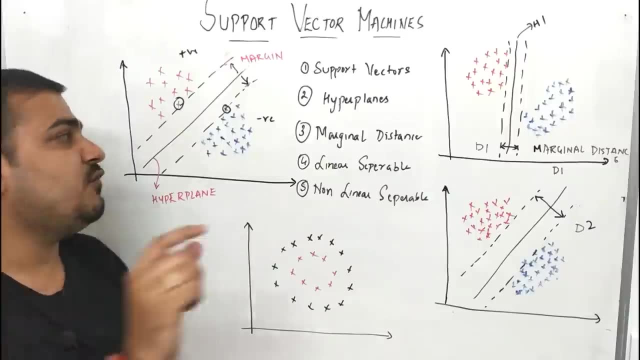 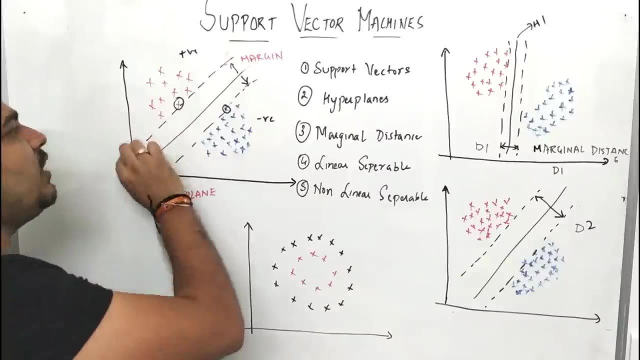 passes through the nearest you know negative point. from there we will actually create this particular hyperplane. That is the intuition behind support vector machine. So support vector machine does not just only focus on creating one hyperplane, but instead it also creates two parallel hyperplanes in such a way that one of the hyperplanes will be passing. 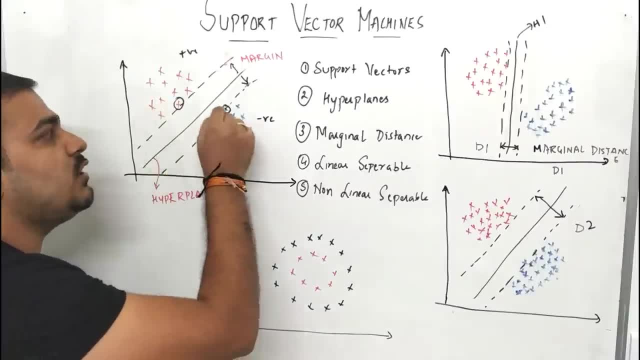 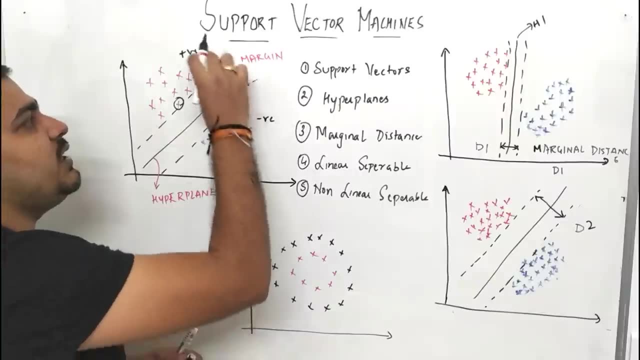 to the nearest positive point and the other hyperplane will be passing to the nearest negative point. Now, when we compute this distance, that is d positive and d minus, this whole distance is basically called as margin Marginal distance. Okay, This dotted line we can consider. 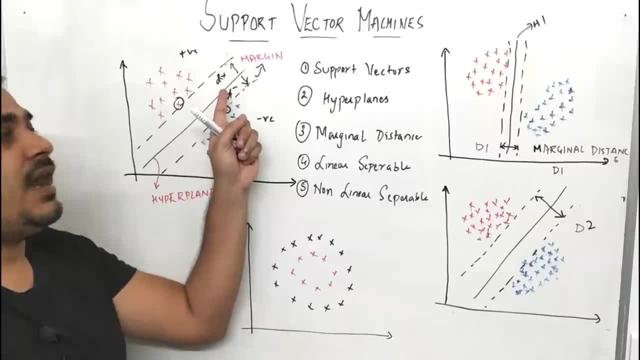 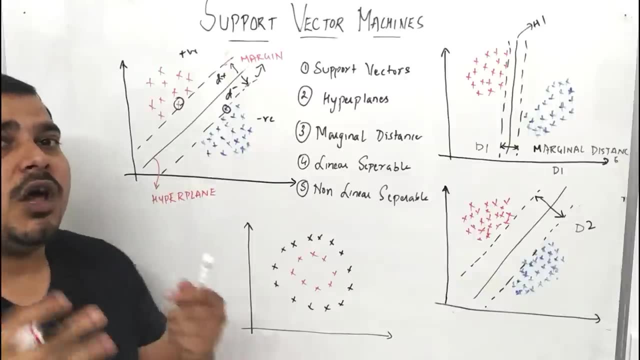 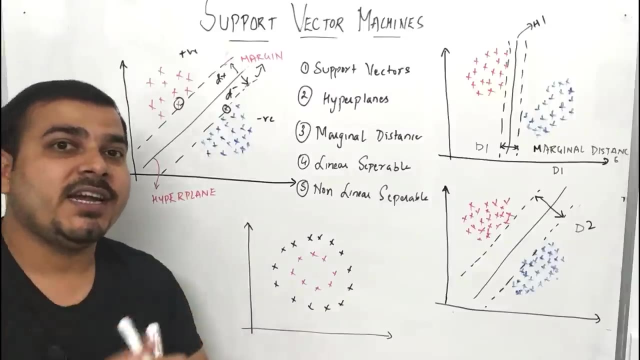 it as margin, and the distance between these two parallel lines, you know, in the dotted line, is called as margin. Now what is the significance of this particular margin? Remember, guys, we always have to create a generalized model. You know, whenever we are applying a classification problem statement, we always have to create a generalized model. Now, in 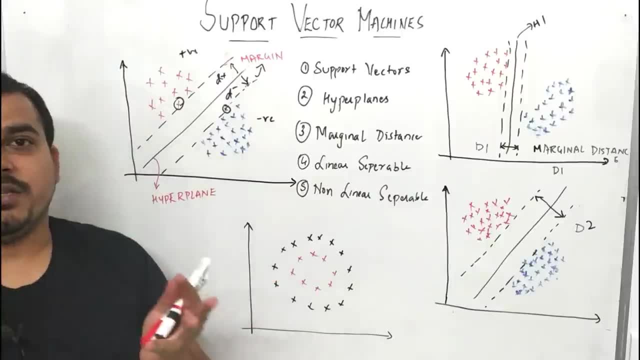 the generalized model. you know, we usually get a better accuracy for any kind of data that we are applying. So we usually get a better accuracy for any kind of data that we actually get. Now, when we are doing this separation with respect to the positive and 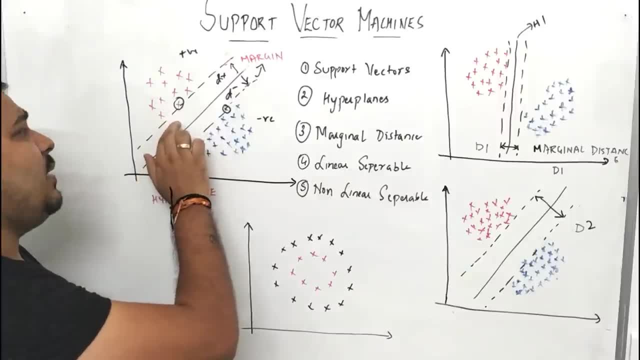 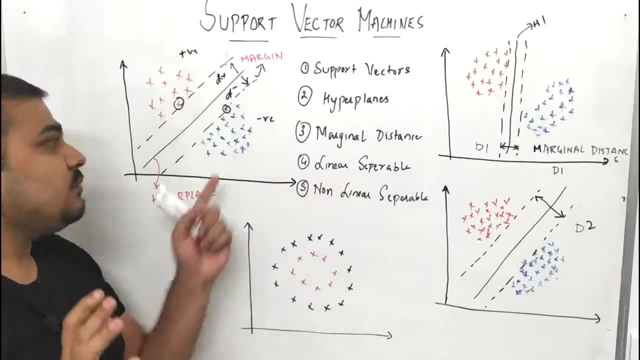 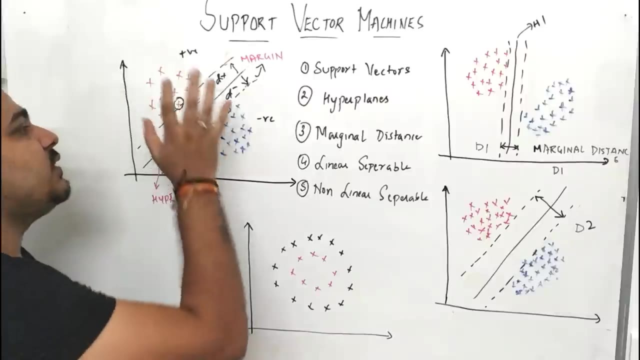 negative. you know, any points, any points that come above this hyperplane will be actually classified to this particular point. Any point that would be below this particular hyperplane, that will be considered as a negative point. Now this hyperplane is actually giving us a cushion to actually divide this positive and negative in a better way. So in the test, 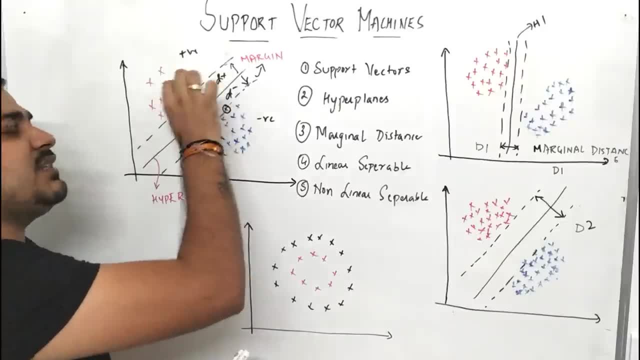 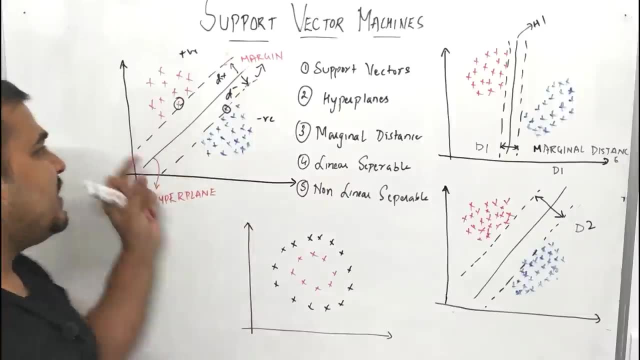 data support. some of the points comes over here. Right, This is just like a cushion which can easily classify And say that, OK, it belongs to the positive class. If it comes away, it belongs to the negative class. So this distance is pretty much important, But still that, the other cushion. 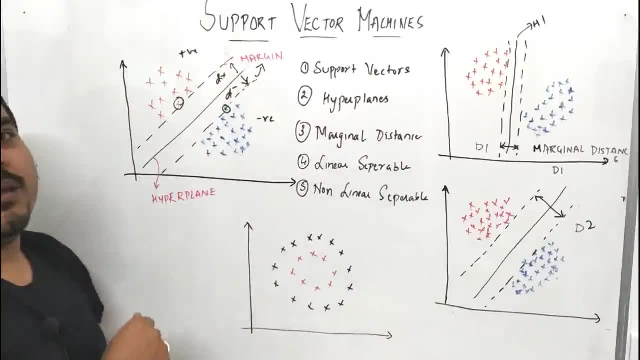 rises that, apart from this hyperplane, we can also create multiple hyperplanes. Right, We can also create some hyperplanes somewhere over here like this: Right, We can create this one single line right, like this, So it is being able to divide this particular points. 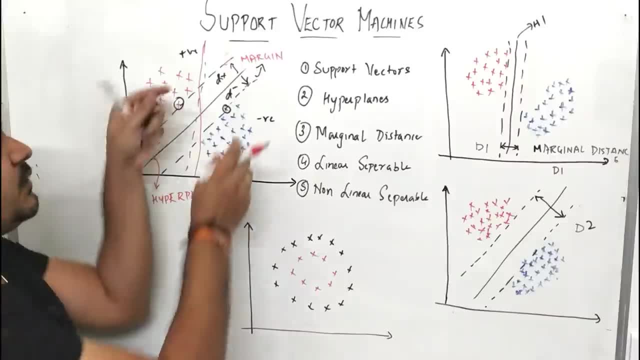 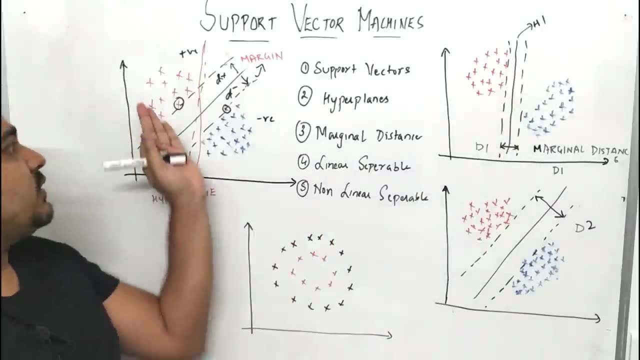 But understand, when I create a hyperplane, I also have to focus on this particular margin. OK, In this particular case, when I'm doing this, I can show you this particular example over here. Right, Suppose I've taken the same points over here and I've actually used this. 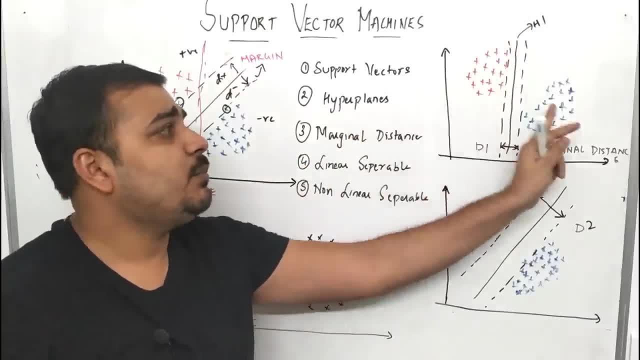 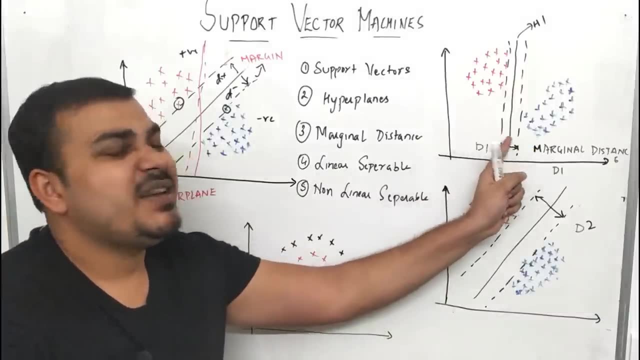 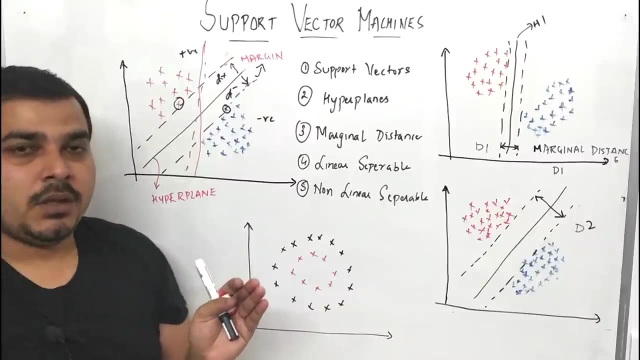 particular hyperplane to actually create a separation line between the positive and the negative class. But when I create this particular marginal planes itself over here, what is happening? this marginal plane distance is very, very less. Our main aim should be that we should maximize this particular marginal plane. OK, So based on that, we actually select the 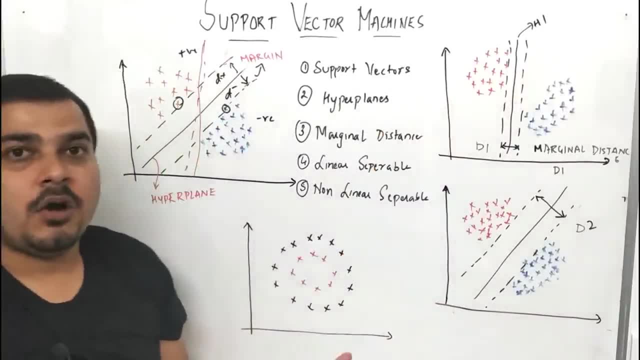 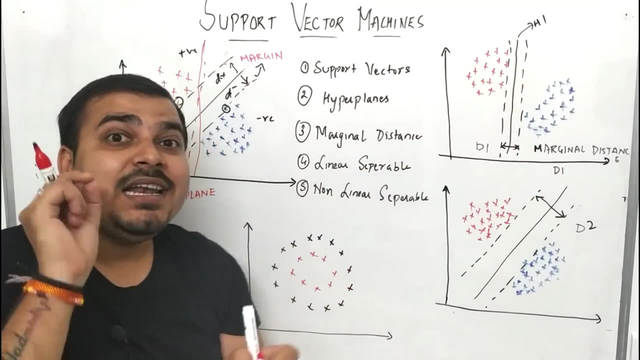 best? hyperplane, What is the maximum marginal plane or marginal distance? you can say: OK, So that is how it is actually. And remember this: all techniques gets applied in linear separable points. You know, over here we can linearly separate this particular point. that basically means we can. 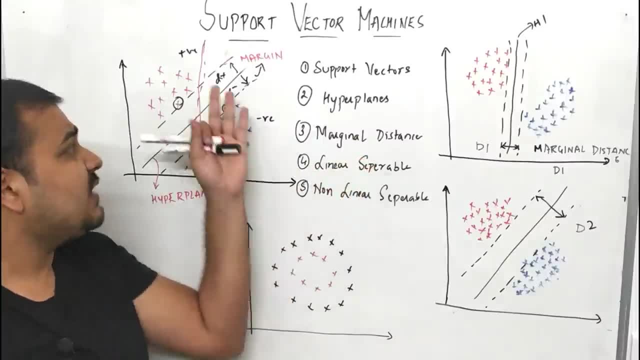 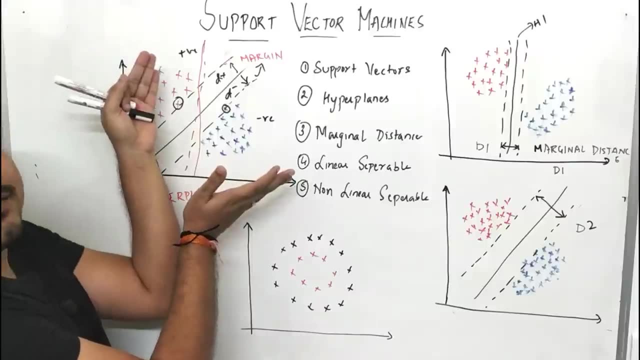 actually create a straight line and we can actually, you know, classify these two points Right. So this linear straight line is basically using, we are using it to actually linearly classify this particular points. What if, if we have nonlinear separable? We'll be discussing. 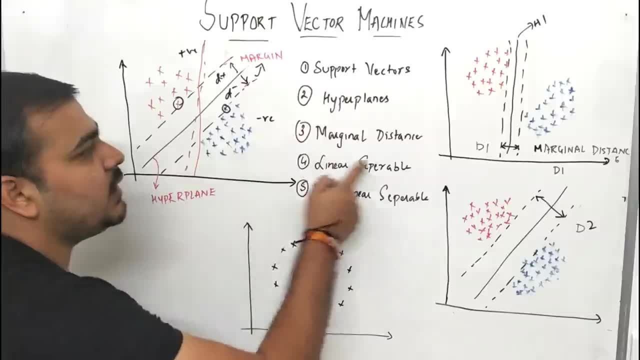 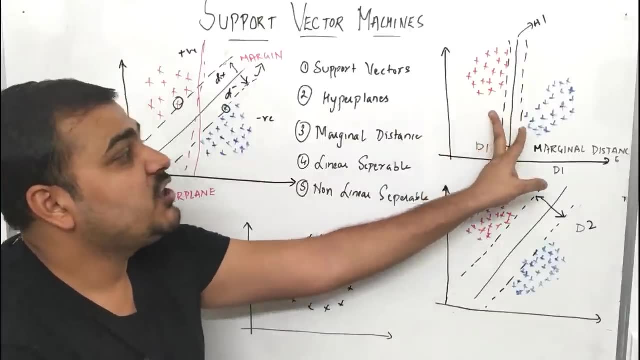 that OK. So the main focus should be that when we are discussing about marginal distance, whenever we create a hyper plane, OK, And those kind of hyper plane should be selected wherein this marginal distance should be maximum. So, if I take this two particular example, one way I've actually used this for linearly separate. 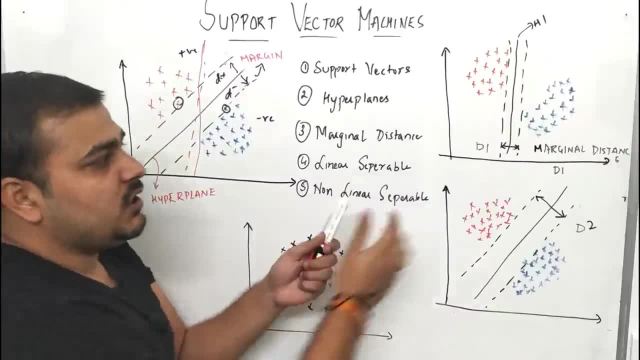 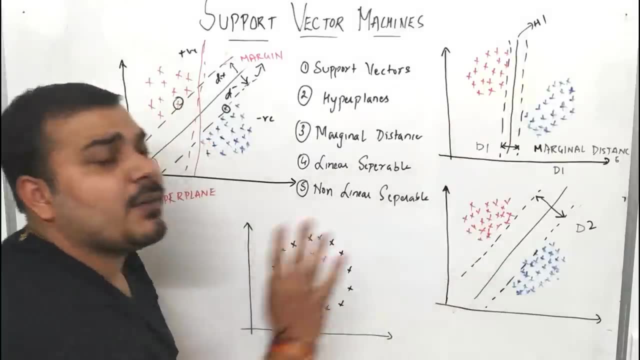 separating in this particular way and the other way, somewhere over here, at this particular distance, I can say it as D 1, this particular distance, I can say it as D2.. Now, in this particular level, which of those particular hyper plane will get selected, whether this one or this? 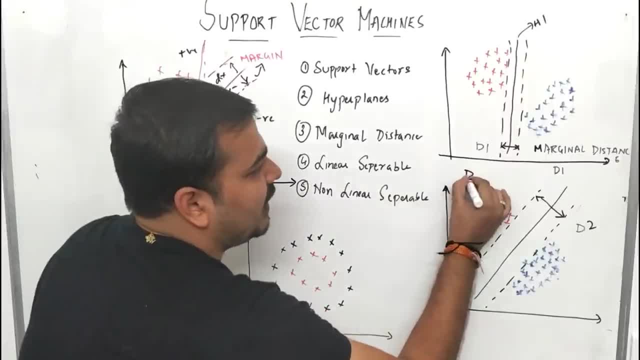 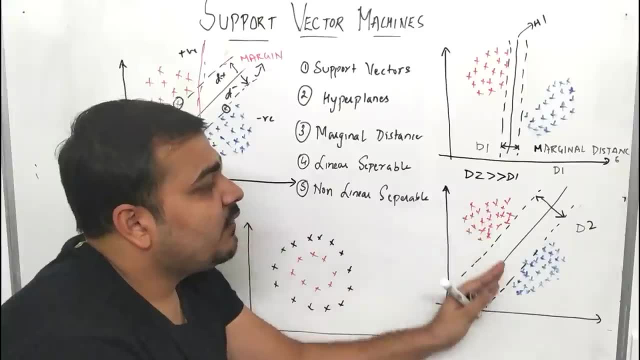 right along with this marginal plane. so definitely over here you can see that the d2 is very, very much greater than what d1. so we may basically use this particular technique to actually divide this, or use this hyperplane to actually divide this particular points, because now here we get a more. 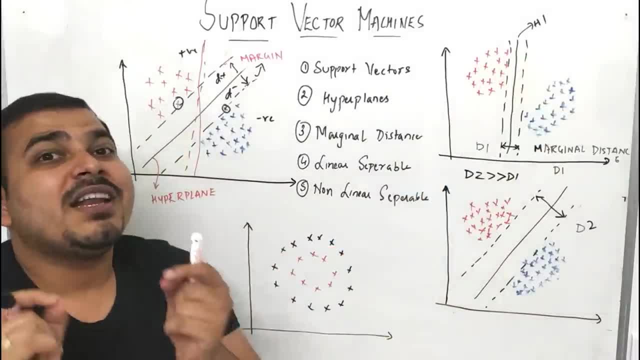 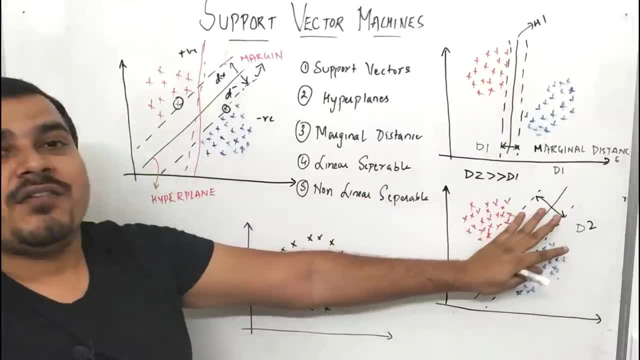 generalized model. this will also work well, but we will not get a much generalized model. that basically means for my new test data, this will definitely give a lot of errors when compared to this kind of hyper plane that we have. so going to this, first of all, we have discussed about hyper. 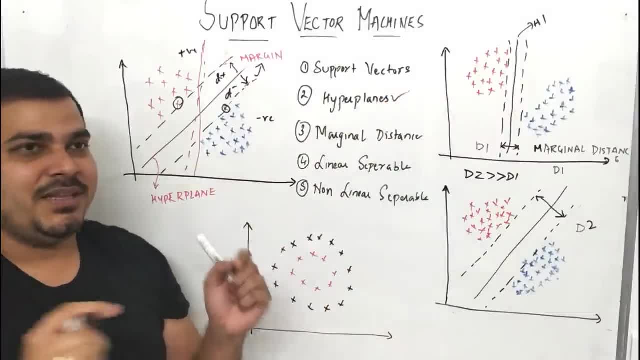 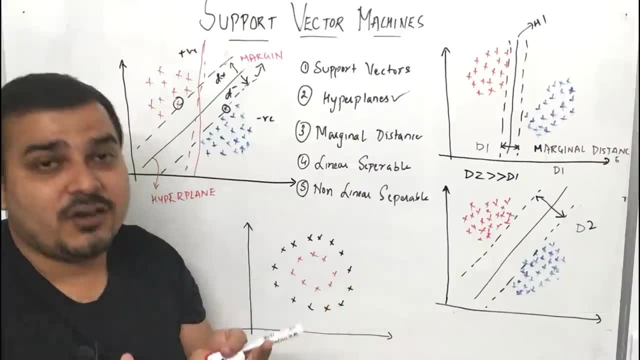 planes. and remember, guys, in two dimension will just not say hyper planes, we'll just say it as a straight line, ok. but in 3 dimensions, in four dimensions, we may say it as a hyper plane because we will be using a kind of planes over there to actually divide those points. ok, so we have. 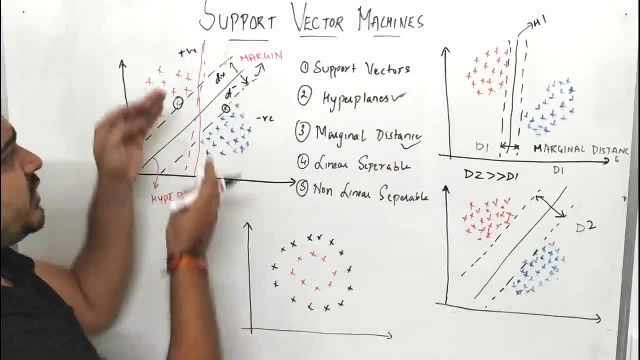 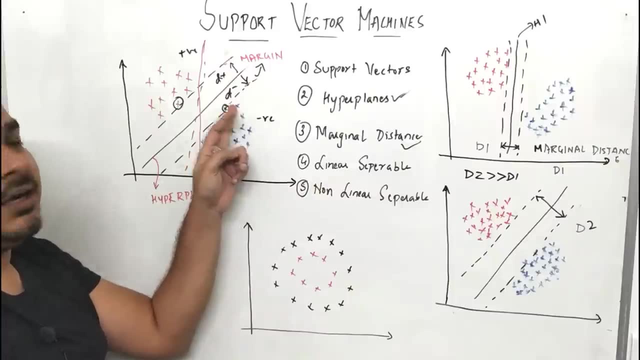 discussed about hyper plane. we have discussed about marginal distance. marginal distance is nothing but the two parallel lines that I am actually creating with respect to the most nearest positive point and the most nearest negative point. the distance between them is actually the marginal distance. this I can say it as: 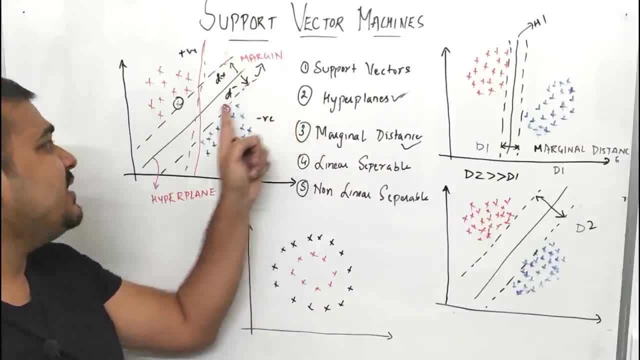 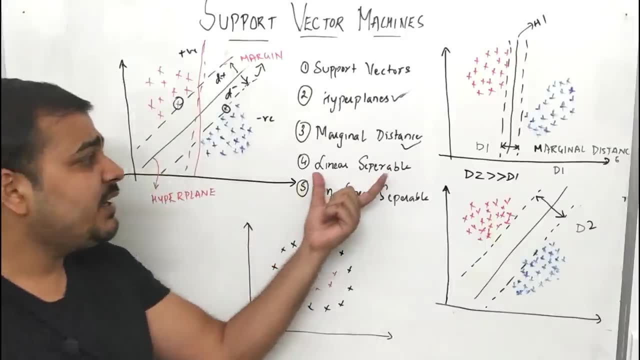 a marginal positive plane, marginal negative plane, because this is nearest to the negative and the positive point. so these two topics have been covered. now we have also discussed about linearly separable. linearly separable basically means we can easily separate this particular point by just drawing a straight line, okay. nonlinear separable basically means 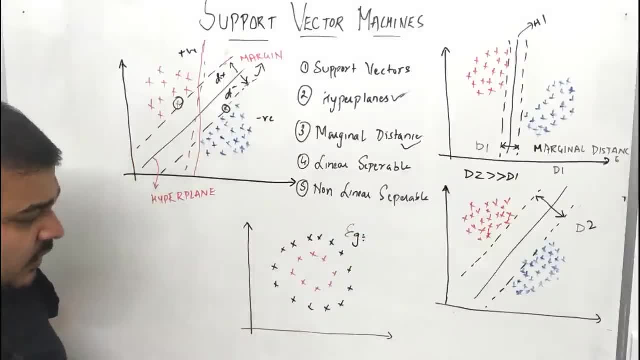 this is the best example. here you can see that we cannot just draw a straight line, right. we cannot just draw a straight line to divide this particular points. anyhow, if we try to do it, our accuracy will be less than 50 percent. less than or equal to 50 percent. right, because 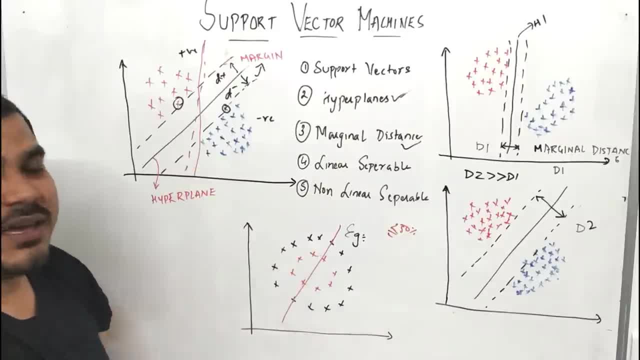 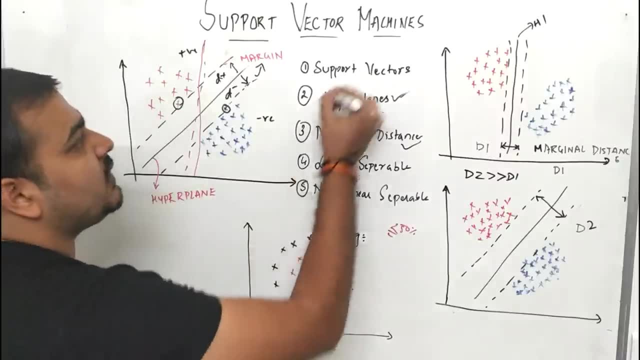 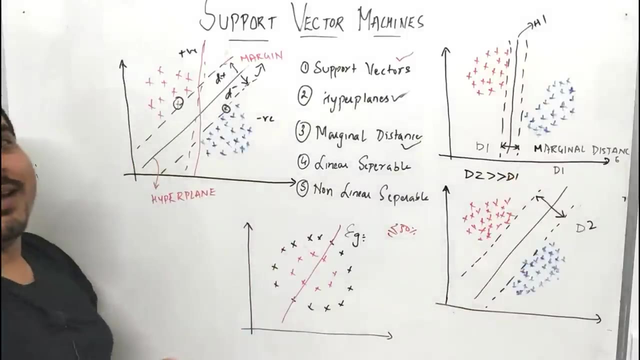 anyhow, you can see, some of the points are over here and some of the points are over here, so they are actually intermixed. so we will also try to understand how to solve this particular problem. okay, now, one important thing is about support vectors. what is this particular support vector? now understand, guys. we have actually created this particular plane. 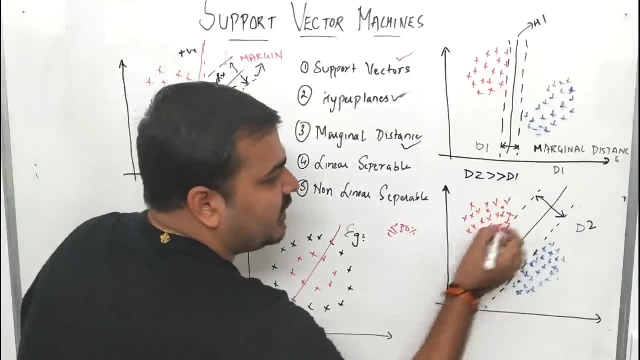 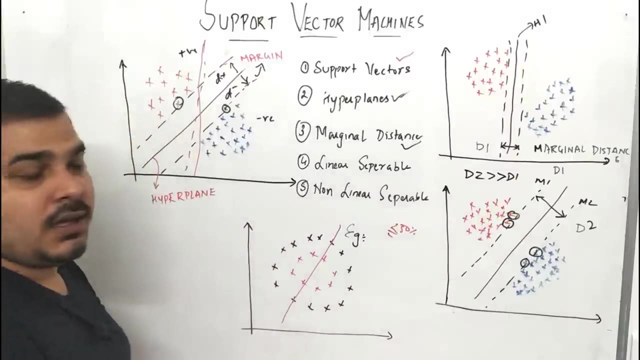 we have selected the maximum distance Now based on this, which is the nearest positive point that is, passing through marginal plane m1 and marginal plane m2, the nearest positive point and the nearest negative point, right, and it may be multiple number of points also. I may have multiple number of points. these 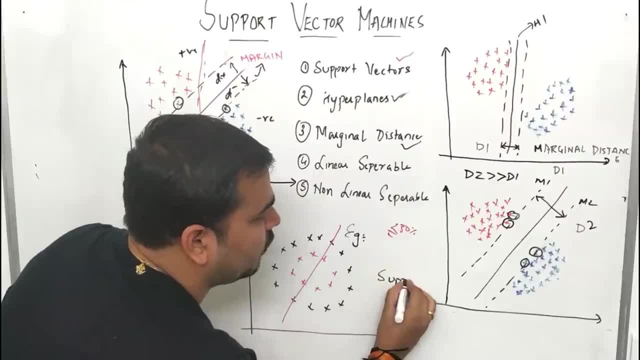 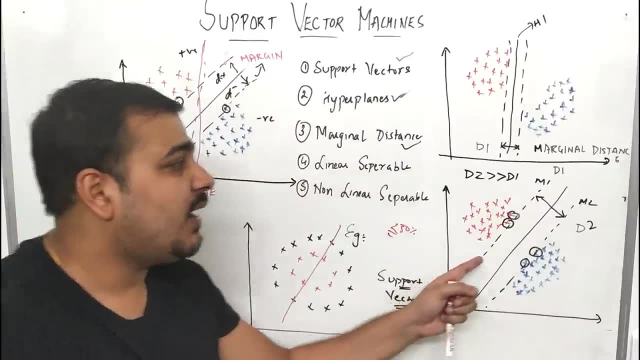 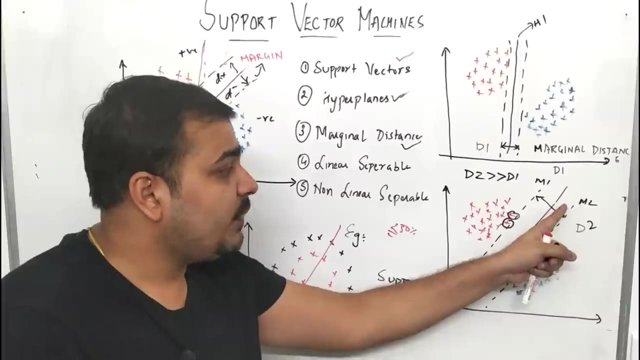 are kind of called as support vectors. so support vectors are nothing but they are the points that is actually passing to the through the marginal plane that we have actually created in parallel to the hyperplane. that is found out right. so based on that and it may be having 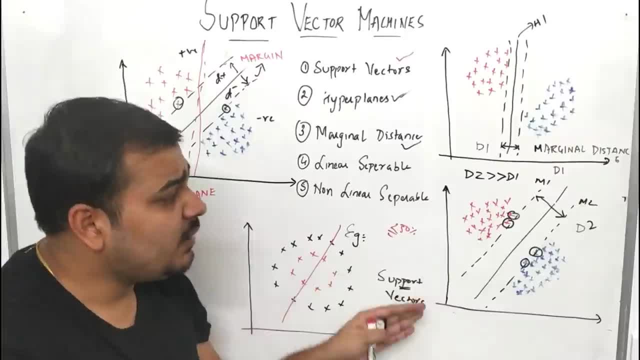 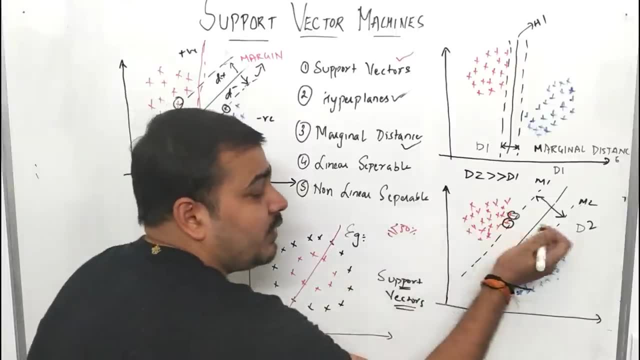 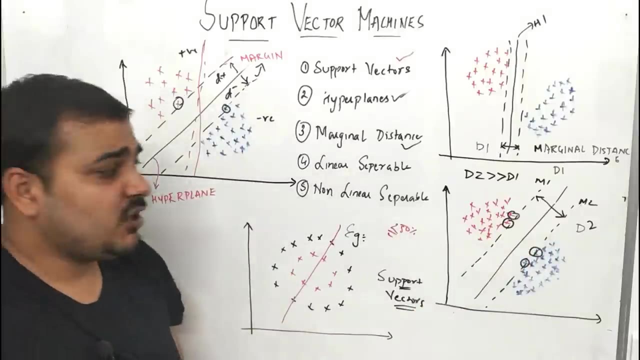 multiple number of points, not one or two, it may be three or four, any number of points that are passing through this particular marginal plane. we will be considering those, as you know. we will be considering those as support vectors. so this is my support vector, this is my support vector, and these all are also pretty much important, guys, because this helps. 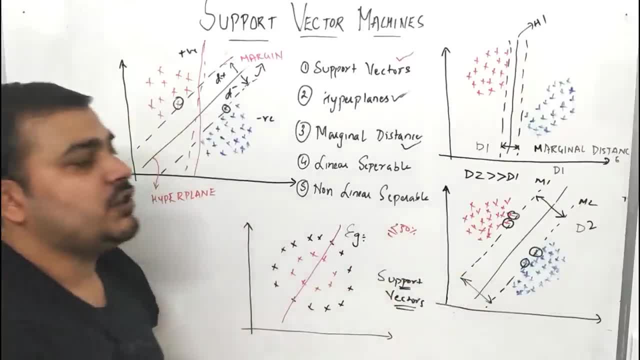 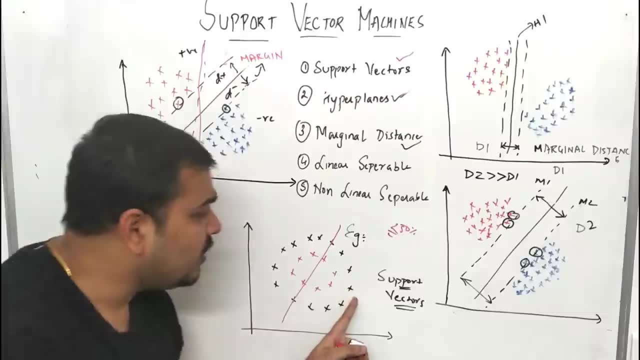 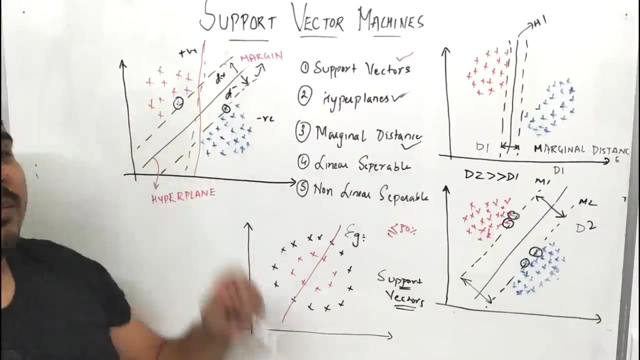 us to determine the maximum distance of the marginal plane. and remember, finally, we have to create a generalized model. now still one question basically arises: how do we solve this kind of problem? statement, and remember, guys, this hyperplane, you know how it is actually getting created. with respect to the hyperplane I will also be discussing in the upcoming 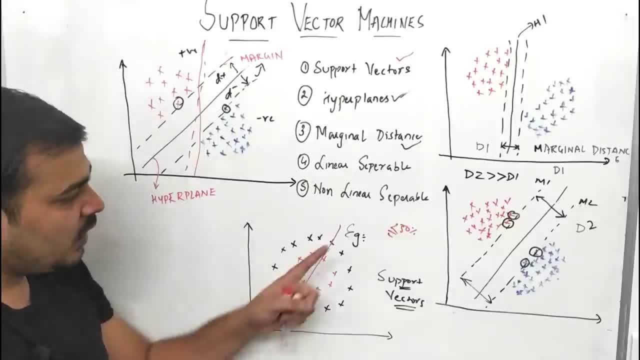 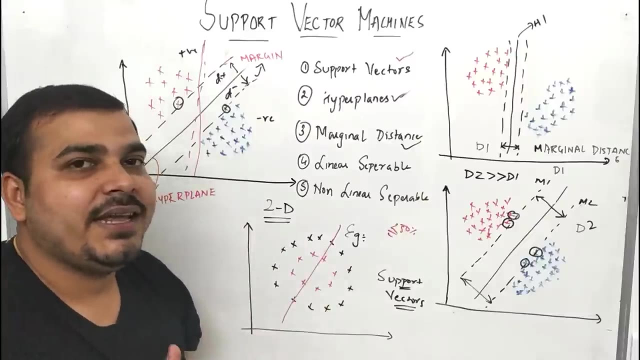 parts now, but still we did not understand how do we solve this kind of problem? remember, this is a two dimensional graph, right, two dimensional graph with respect to the positive and the negative statement. so I can, I can. in order to solve this support vector machine uses a technique called as SVM kernels. now, this SVM kernels, the main aim is that it. 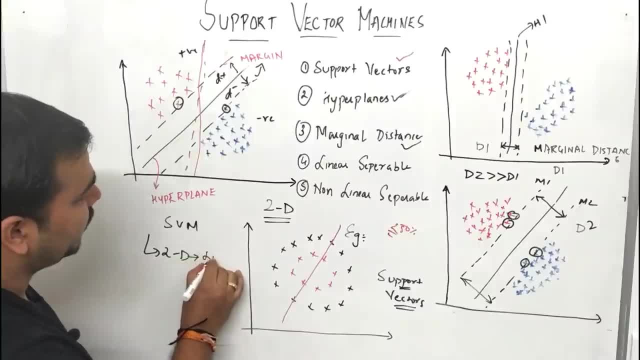 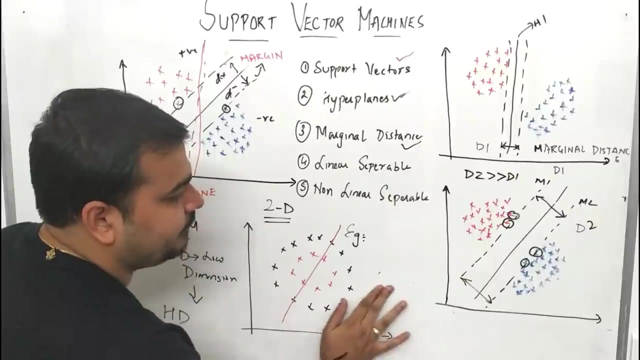 tries to convert the two dimensional- I'll say low dimension, low dimension- into a high dimension. okay, now, what do I mean by high dimensions? just take this particular example, guys. I'm just going to rub this so that you'll be able to understand. okay, suppose, if I consider: 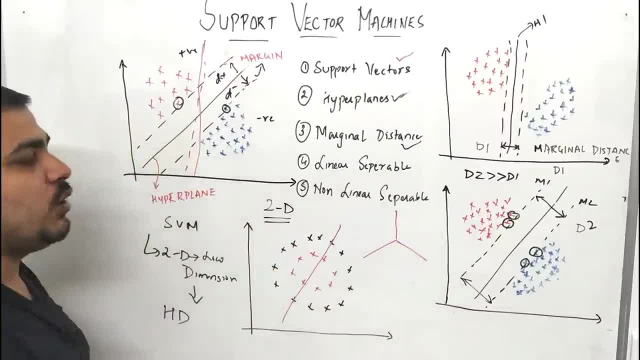 a three dimensional graph And if I try to convert this two dimension into three dimension, so okay, suppose some of the points of my black points are over here, right, and if I convert this into three dimension I can actually create a hyperplane between this right. so now, when I convert this, 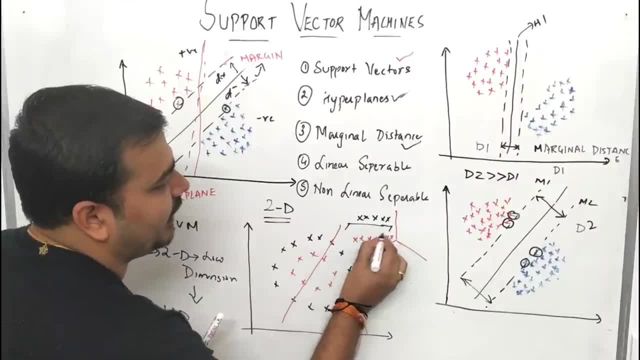 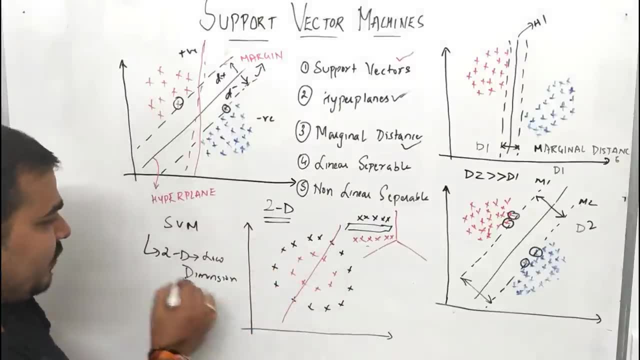 two dimension to three dimension. this will basically get converted like this and between that I can actually create a smaller hyperplane which is basically a conversion. and here what we are doing, we are converting And I'll just name this as SVM kernels. the SVM kernels main aim is actually to convert a lower dimension into a higher. 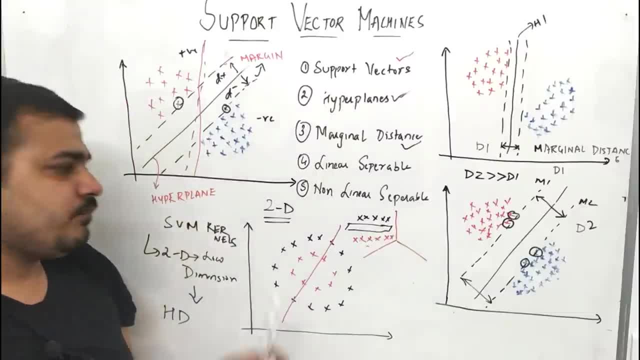 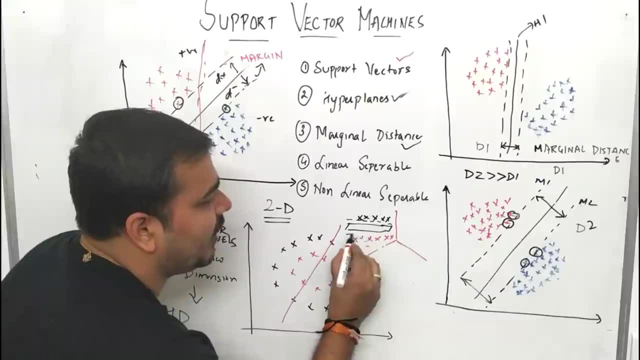 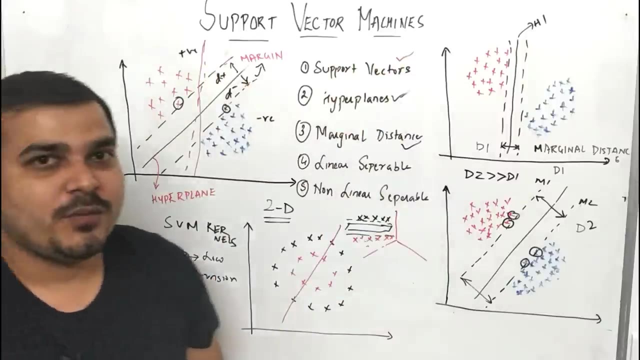 dimension, so that we will be easily able to, you know, classify this particular points by a hyperplane itself. okay, and with respect to this hyperplane also, I'll be getting my marginal plane, which looks like this and it will be easily separable. but still understand, guys, we have just understood the basic understanding of support vector machines in the future class. 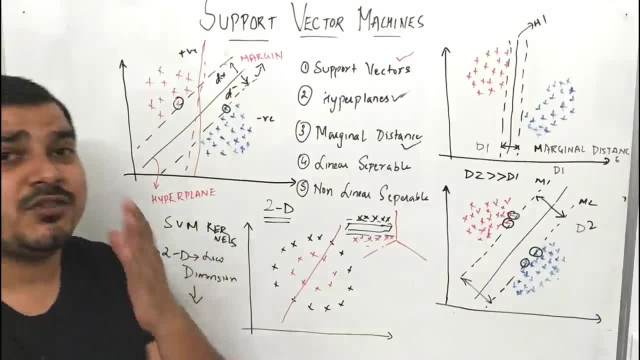 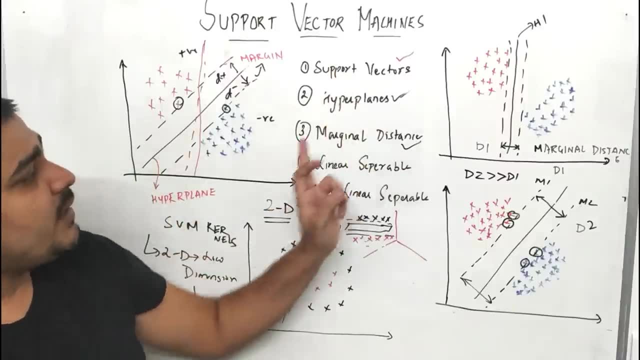 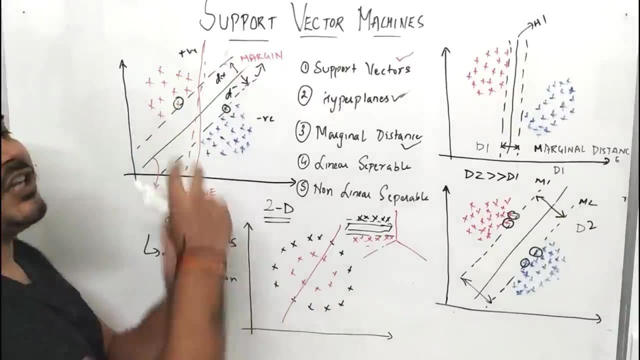 we'll also be discussing about a lot of maths thing, about SVM kernels, different types of SVM kernels, but I hope you have understood- please do remember this- particular terminologies, that is, support vectors, hyperplane, marginal distance, linearly separable, non-linear separable. again, understand that our main aim is to create a generalized model by just not creating a 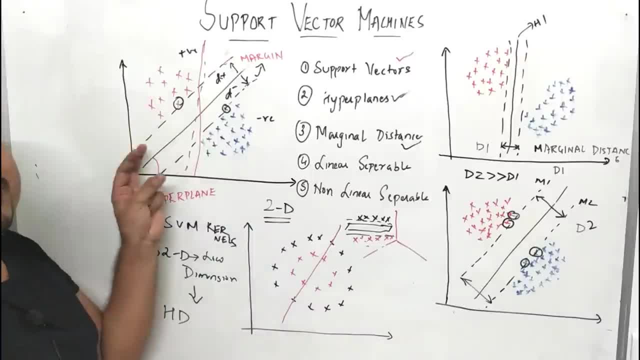 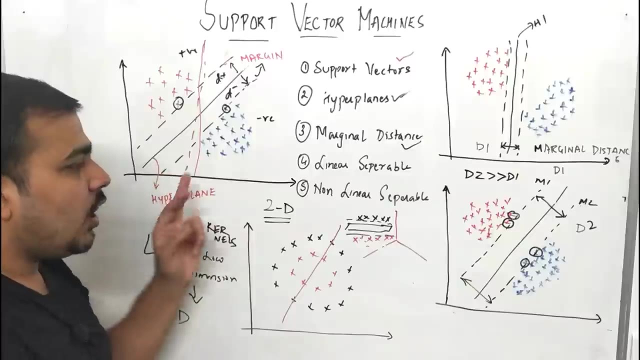 hyperplane, but instead we are creating a marginal distance, you know, with respect to the marginal planes that are created with respect, again, with respect to the positive and the negative points, right. So the higher the marginal distance, The more generalized our model is, but definitely this will not be possible with respect to 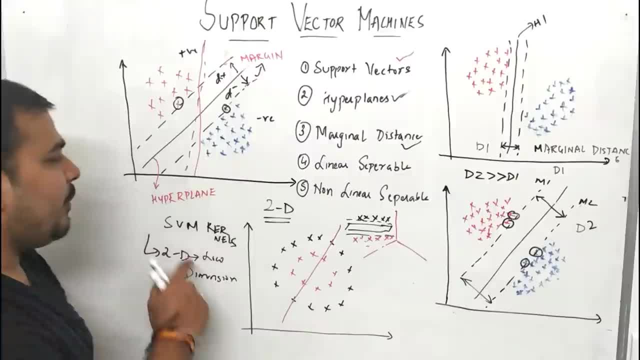 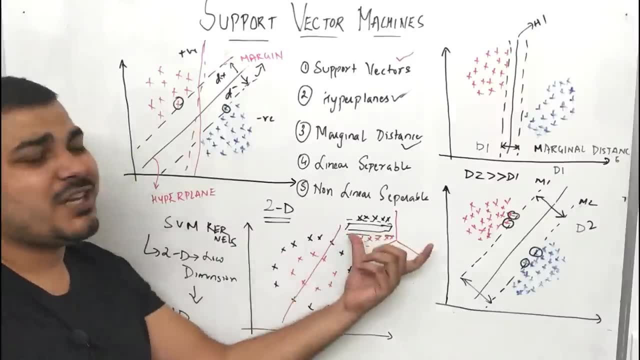 this kind of non-linear, separable points. for this we usually apply SVM kernels, where in we convert our low dimension into high dimension and lower dimension. it may be like two dimension to three dimension or two dimension to four dimension, by creating new data points, or we'll 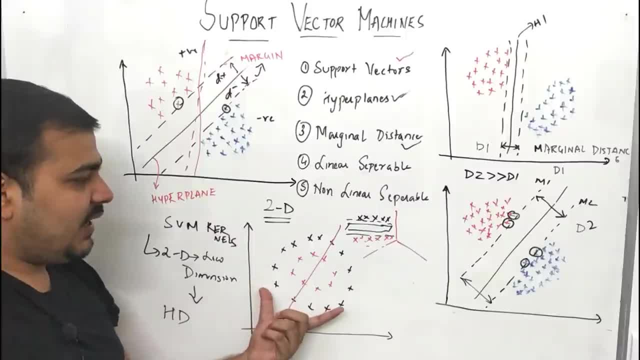 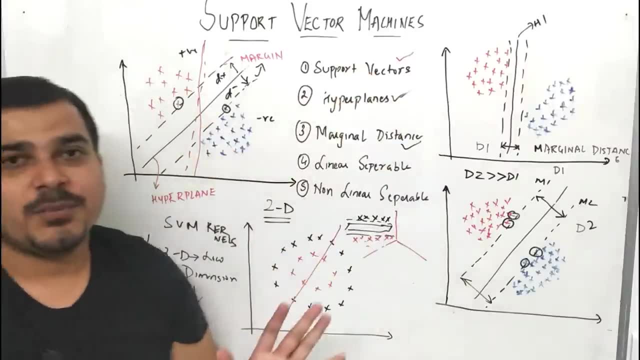 try to, you know, move it in this particular way. now, here you can see that this two dimension is getting converted into three dimension easily. we can actually create a hyperplane with respect to the positive and negative points and we can actually create a non-linear, separable point. 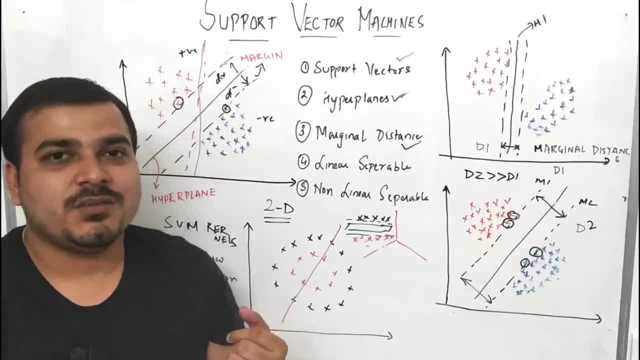 So this is the understanding of support vector machines. in the upcoming classes I'll be discussing about a lot of maths, how to actually apply this, SVM kernels, what are the different SVM kernels? but just go through this, read a lot of blocks and try to understand and yes, I'll